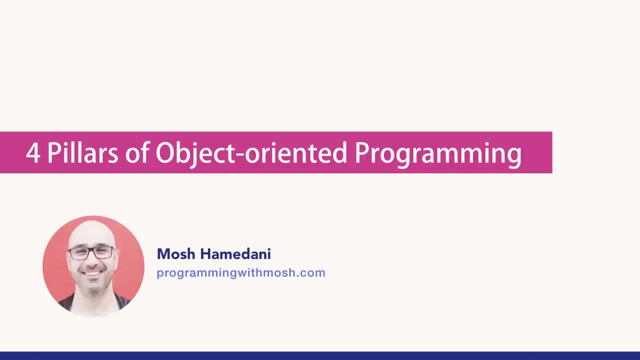 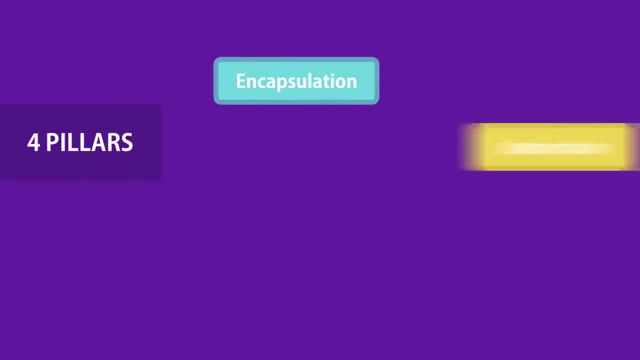 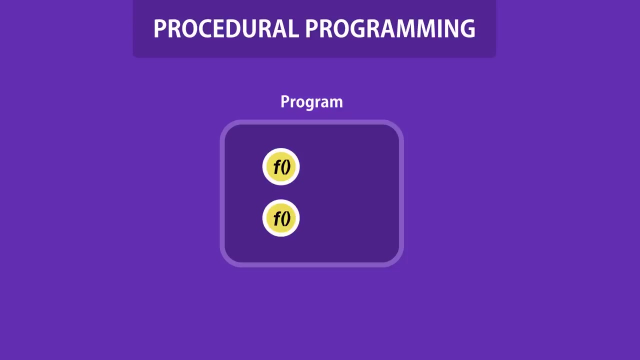 A popular interview question concerns the four core concepts in object-oriented programming. These concepts are encapsulation, abstraction, inheritance and polymorphism. Let's look at each of these concepts. Before object-oriented programming we had procedural programming that divided a program into a set of functions, So we have data stored in a bunch of variables. 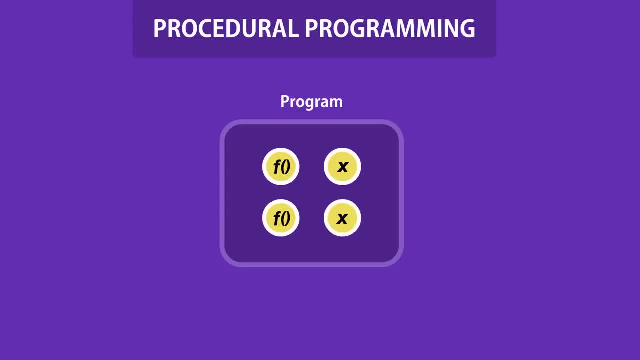 and functions that operate on the data. This style of programming is very simple and straightforward. Often it's what you will learn as part of your first programming subject at a university, But as your programs grow, you will end up with a bunch of functions that are all over the place. 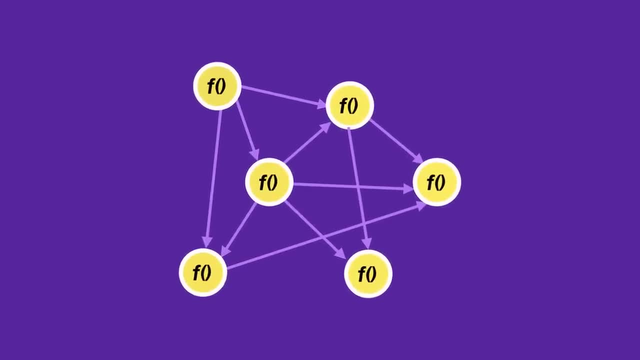 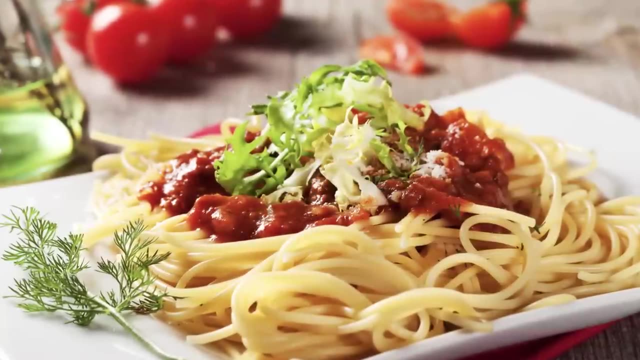 You might find yourself copying and pasting lines of code over and over. You make a change to one function and then several other functions break. That's what we call spaghetti code. There is so much interdependency between all of these functions. There is so much interdependency between all of 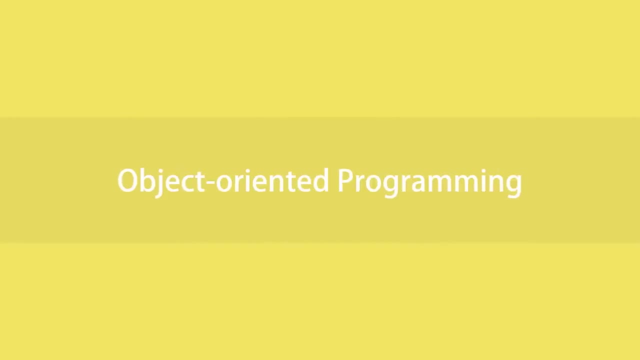 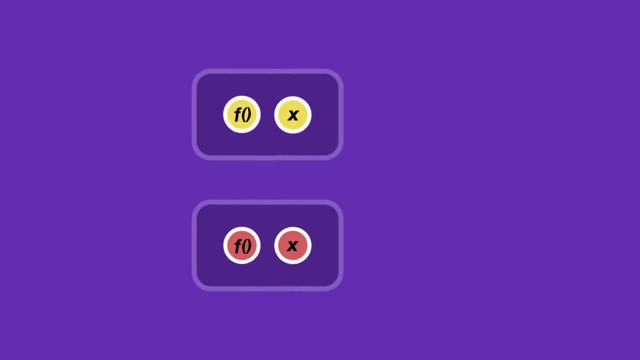 these functions, it becomes problematic. Object-oriented programming came to solve this problem. In object-oriented programming we combine a group of related variables and functions into a unit. We call that unit an object. We refer to these variables as properties and the functions. 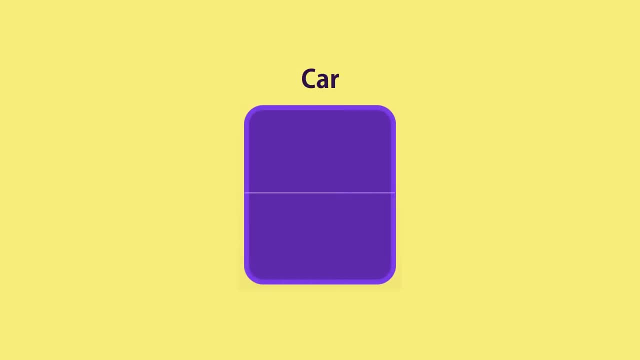 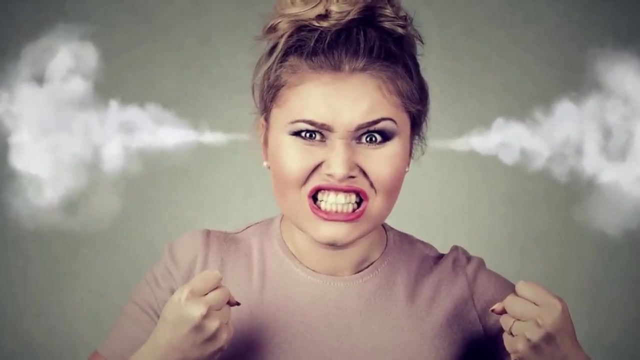 as methods. Here is an example. Think of a car. A car is an object with properties such as make, model and color, and methods like start, stop and move. now you might say: what mosh? we don't have cars in our programs. give me a real programming. 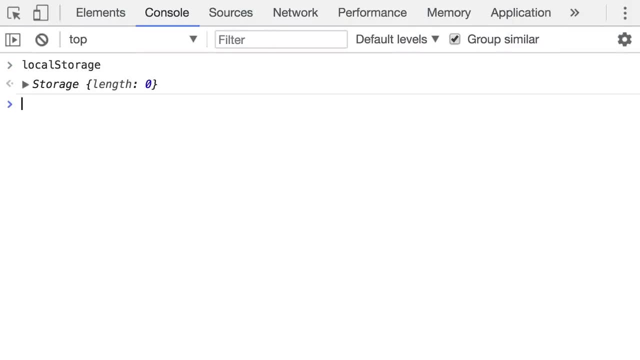 example. okay, think of the local storage object in your browsers. every browser has a local storage object that allows you to store data locally. this local storage object has a property like length, which returns the number of objects in the storage, and methods like set item and remove item. so in 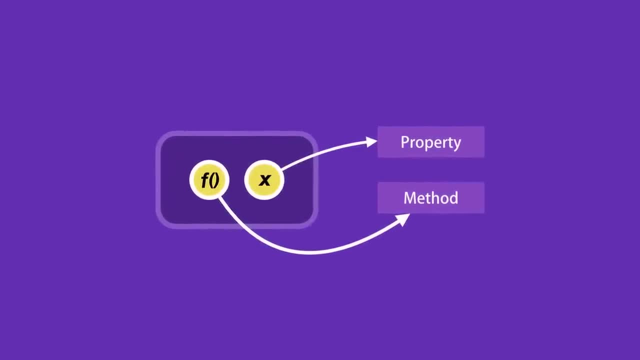 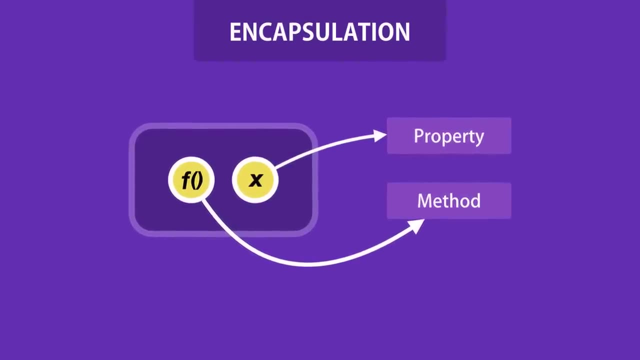 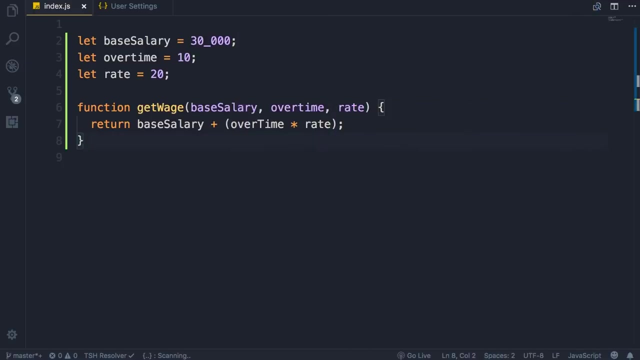 object-oriented programming. we group related variables and functions that operate on them into objects, and this is what we call encapsulation. let me show you an example of this in action. so here we have three variables: base salary, overtime and rate. below these we have a function to calculate the wage for an employee. we refer to this kind of implementation as procedural, so we 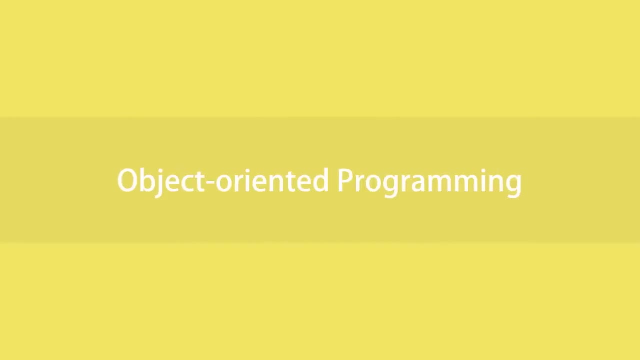 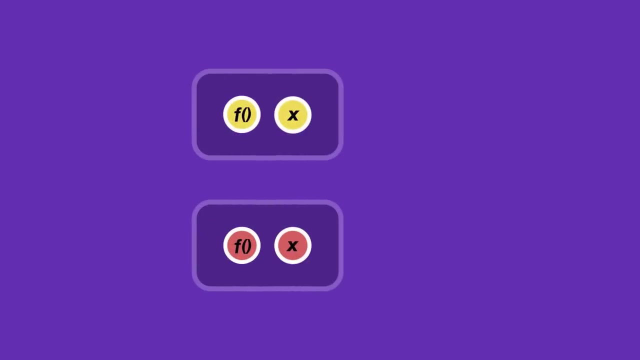 these functions, It becomes problematic. Object-oriented programming came to solve this problem. In object-oriented programming we combine a group of related variables and functions into a unit. We call that unit an object. We refer to these variables as properties and the functions. 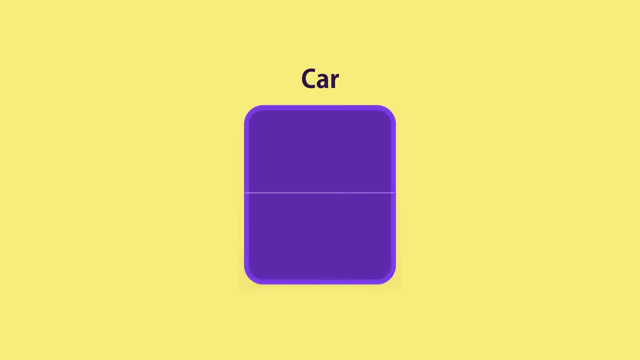 as methods. Here is an example. Think of a car. A car is an object with properties such as make, model and color, and methods like start, stop and move. Now you might say: but Mosh, we don't have cars in our programs. Give me a real. 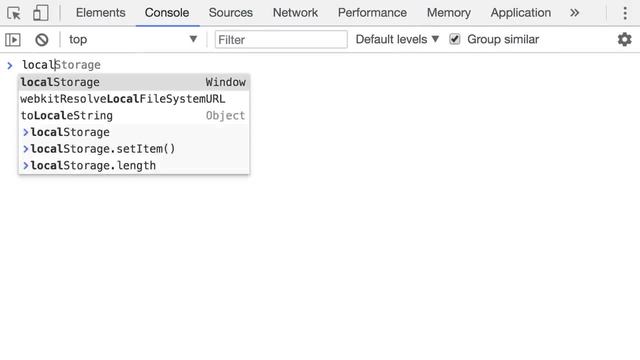 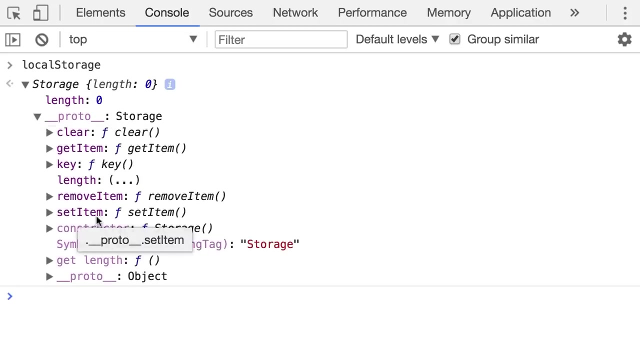 programming example. Okay, think of the local storage object in your browsers. Every browser has a local storage object that allows you to store data locally. This local storage object has a property like length, which returns the number of objects in the storage, and methods. 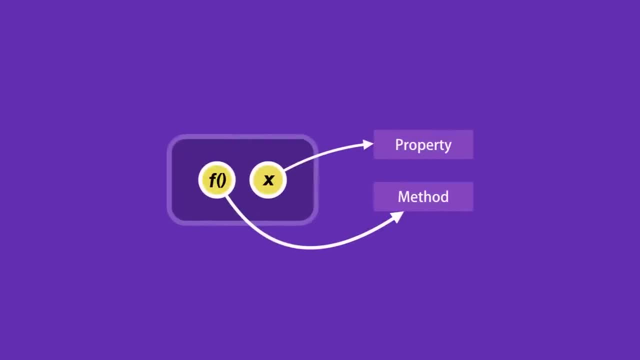 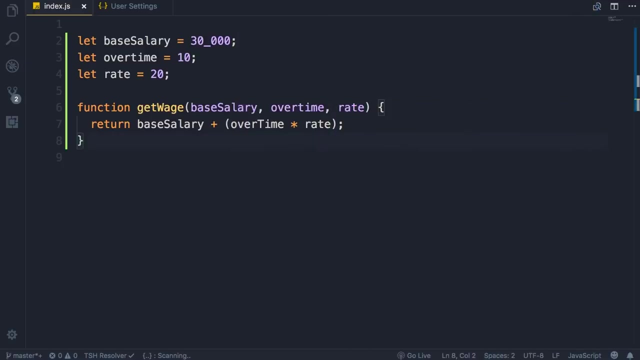 like set item and remove item. So in object-oriented programming we group related variables and functions that operate on them into objects, And this is what we call encapsulation. Let me show you an example of this in action. So here we have three variables: base salary. 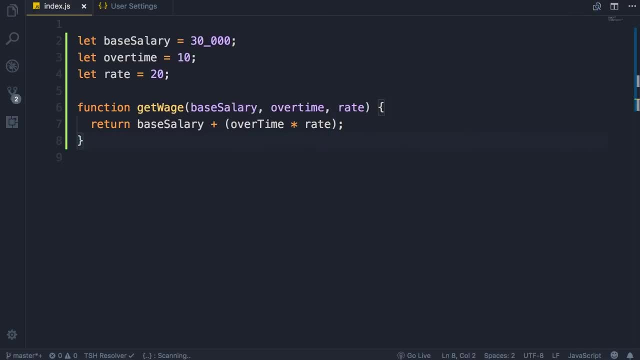 overtime and rate. Below these, we have a function to calculate the wage for an employee. We refer to this kind of implementation as procedural. So we have variables on one side and functions on the other side. They are decoupled. Now let's take a look at the object-oriented 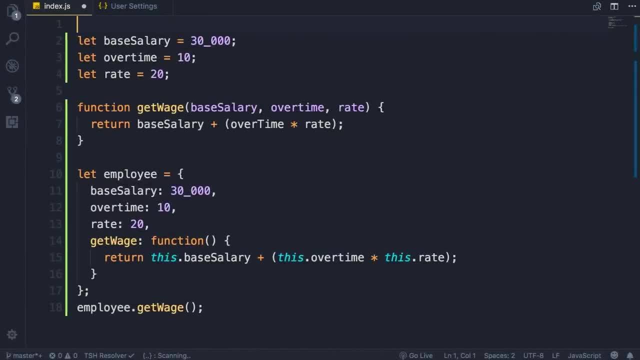 way to solve this problem. We can have an employee object with three properties- base salary, overtime and rate- and a method called getWage. Now, why is this better? Well, first of all, look at the getWage function. This function, 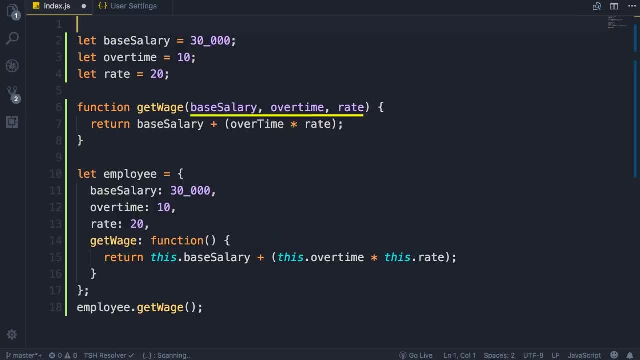 has no parameters. In contrast, in a procedural example, our getWage function has three parameters. The reason, in this implementation, we don't have any parameters is because all of these parameters are actually modeled as properties of this object: All these properties and the getWage function. 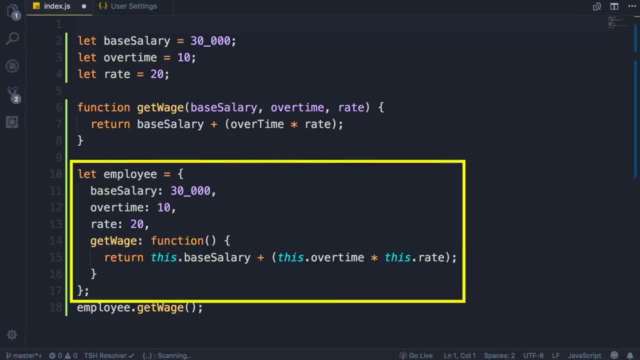 they are highly related, so they are part of one unit. So one of the symptoms of procedural code is functions with so many parameters. When you write code in an object-oriented way, your functions end up having fewer and fewer parameters, As Uncle Bob says. 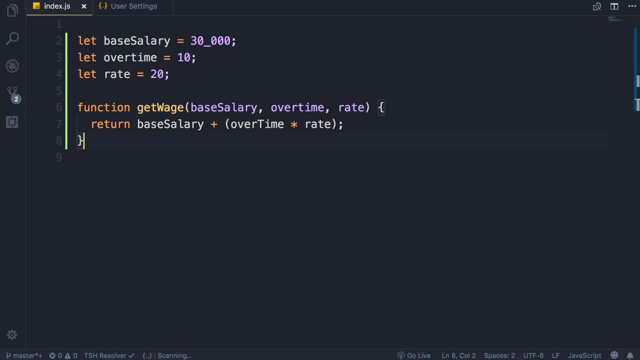 have variables on one side and functions on the other side. they are determined, coupled. now let's take a look at the object-oriented way to solve this problem. we can have an employee object with three properties- base salary, overtime and rate- and a method called get wage. now why is this better? well, first of all, look at the get wage function. this function has: 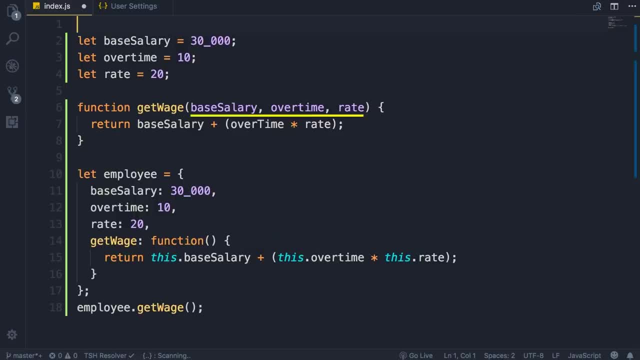 no parameters. in contrast, in a procedural example, our get wage function has three parameters. the reason in this implementation we don't have any parameters is because all these parameters are actually modeled as properties of this object, all these properties and the get wage function. they are highly related, so they are part of one unit. 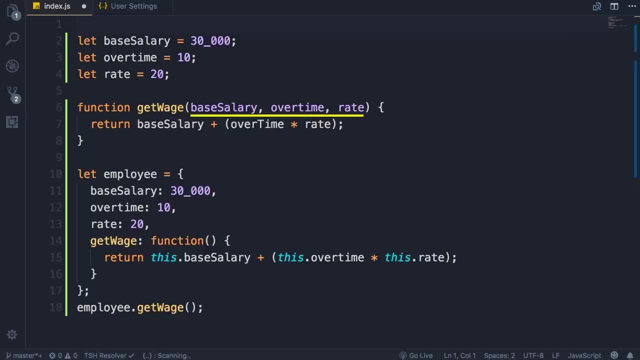 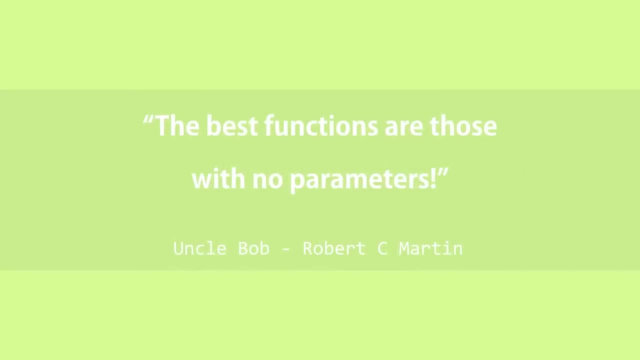 so one of the symptoms of procedural code is functions with so many parameters. when you write code in object-oriented way, your functions end up having fewer and fewer parameters. as uncle bob says, the best functions are those with no parameters. the fewer the number of parameters, the easier it is to use and maintain that function. so that's encapsulation. now let's. 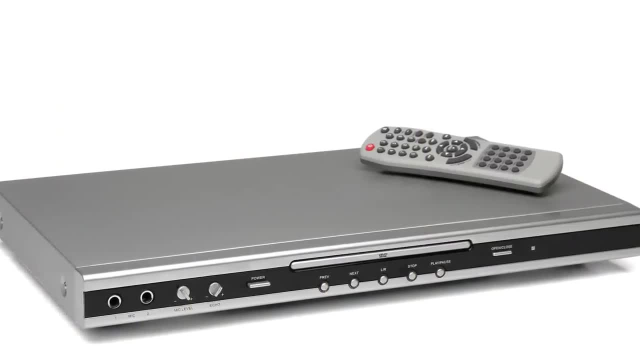 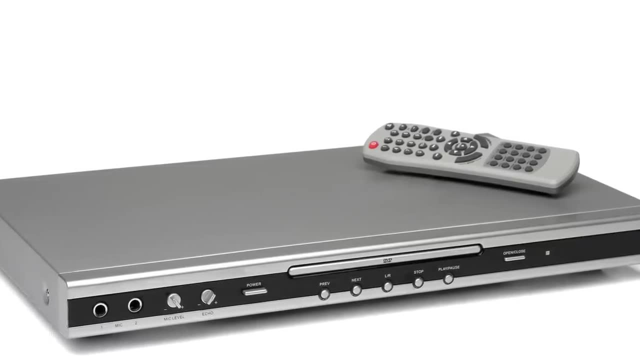 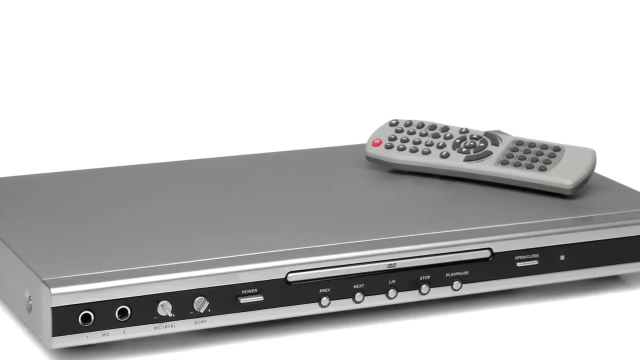 look at abstraction. think of a dvd player as an object. this dvd player has a complex logic board on the inside and a few buttons on the outside that you interact with. you simply press the play button and you don't care what happens on the inside. all that complexity is hidden from you. 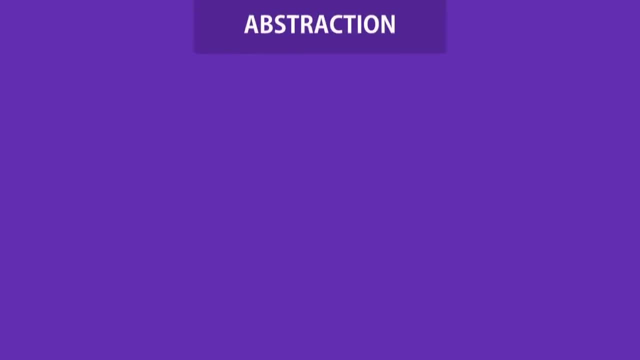 this is abstraction. in practice, we can use the same technique in our objects to add new parameters and so on, so we can hide some of the properties and methods from the outside, and this gives us a couple of benefits. first is that we'll make the interface of those 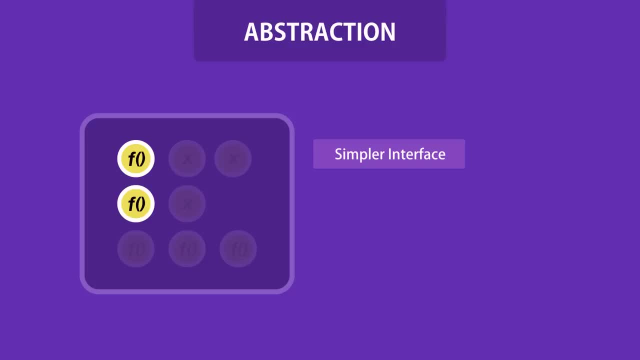 objects simpler. using and understanding an object with a few properties and methods is easier than an object with several properties and methods. the second benefit is that it helps us reduce the impact of change. let's imagine that tomorrow we change, these inner or private methods will leak to the outside, because we don't have any code that touches these. 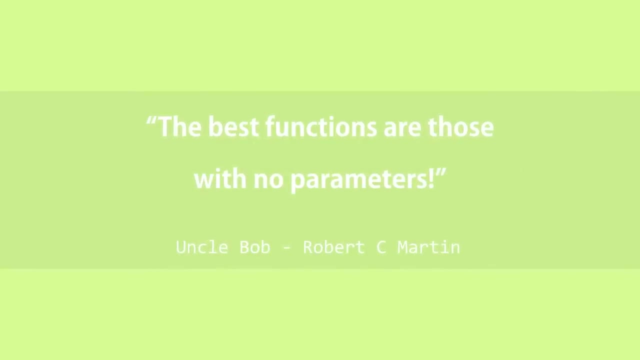 the best functions are those with no parameters. The fewer the number of parameters, the easier it is to use and maintain that function. So that's encapsulation. Now let's look at abstraction. Think of a DVD player as an object. This DVD player, 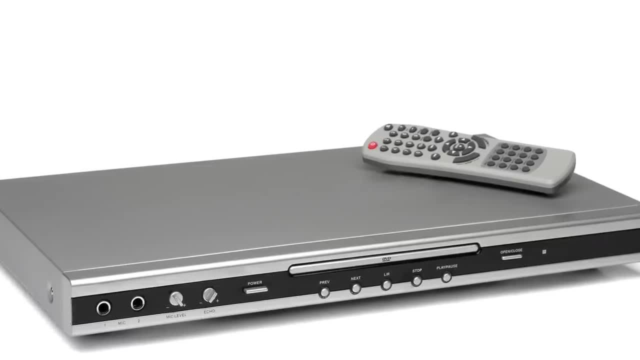 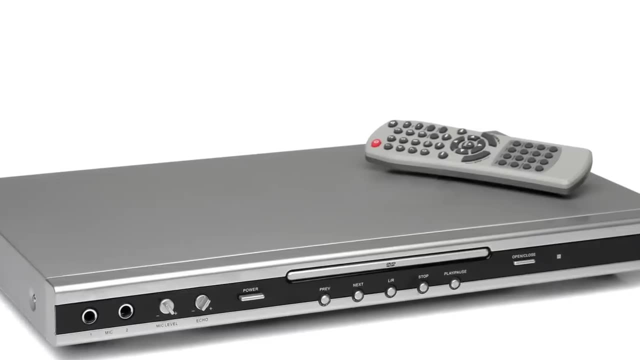 has a complex logic board on the inside and a few buttons on the outside that you interact with. You simply press the play button and you don't care what happens on the inside. All that complexity is hidden from you. This is abstraction in practice. 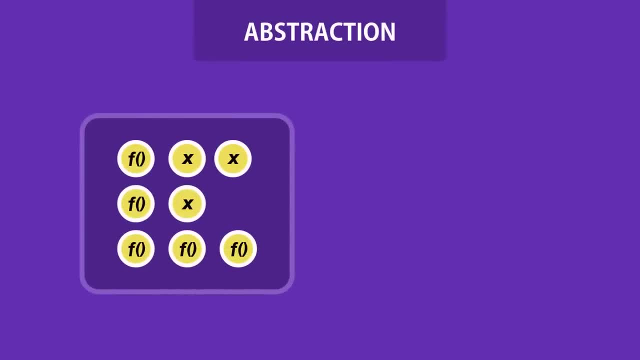 We can use the same technique in our objects, So we can hide some of the properties and methods from the outside, and this gives us a couple of benefits. First is that we'll make the interface of those objects simpler: Using and understanding an object with a few 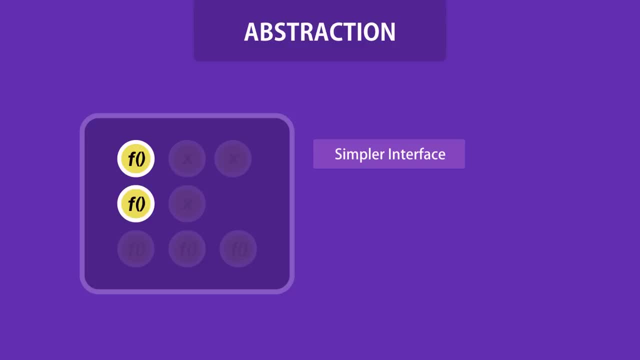 properties and methods is easier than an object with several properties and methods. The second benefit is that it helps us reduce the impact of change. Let's imagine that tomorrow we change these parameters and we'll have a new object. So let's use these inner or private methods. None of these changes will leak. 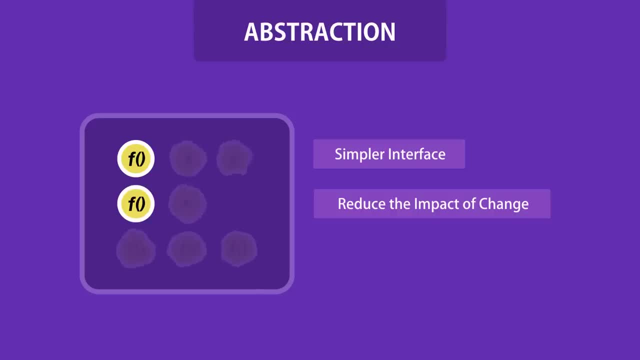 to the outside, because we don't have any code that touches these methods outside of their containing object. We may delete a method or change its parameters, but none of these changes will impact the rest of the application's code. So with abstraction we reduce the. 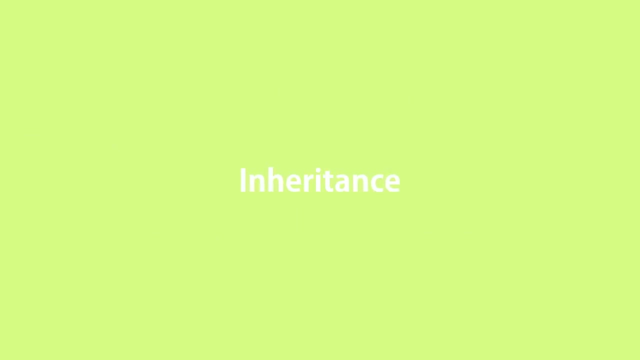 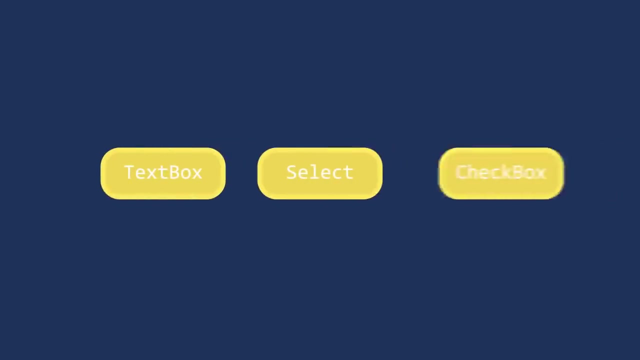 impact of change. Now the third core concept in object-oriented programming: Inheritance. Inheritance is a mechanism that allows us to create a certain type of code and we can use it to create a specific type of code. The three key elements of the HTML element: 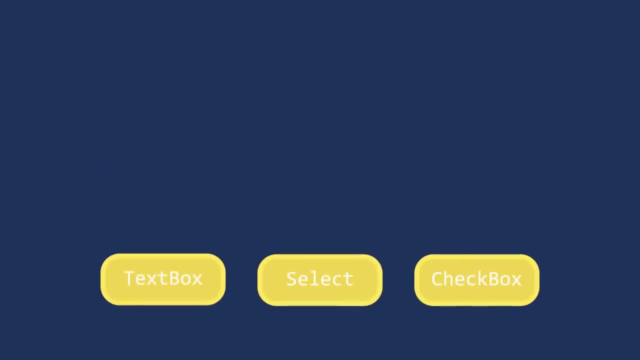 are text boxes, drop-down lists and check boxes. All of these elements have a few things in common. They should have properties like hidden and inner HTML and methods like click and focus, Instead of redefining all of these properties and methods for every type of 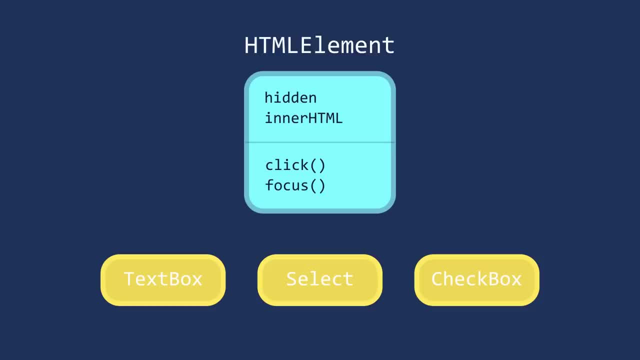 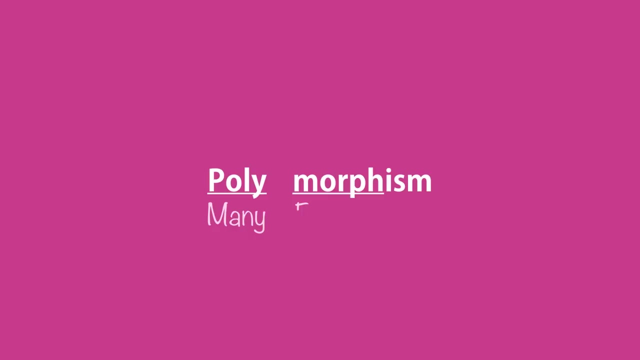 HTML element. we can define them once in a generic object, call it HTML-element and have other objects that we can use to define it. objects inherit these properties and methods, so inheritance helps us eliminate redundant code. and finally, polymorphism: poly means many, morph means form, so polymorphism means 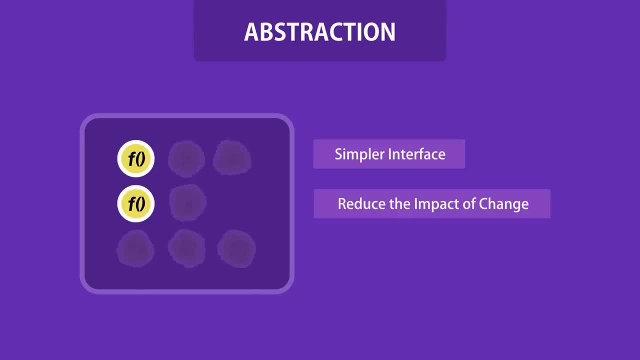 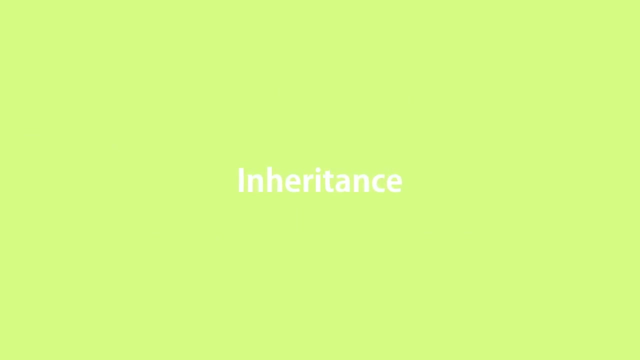 methods outside of their containing object. We may delete a method or change its parameters, but none of these changes will impact the rest of the application's code. So with abstraction we reduce the impact of change. Now the third core concept in object-oriented programming: Inheritance. Inheritance is a mechanism. 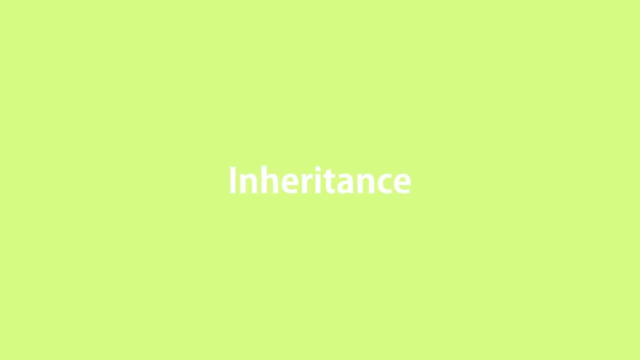 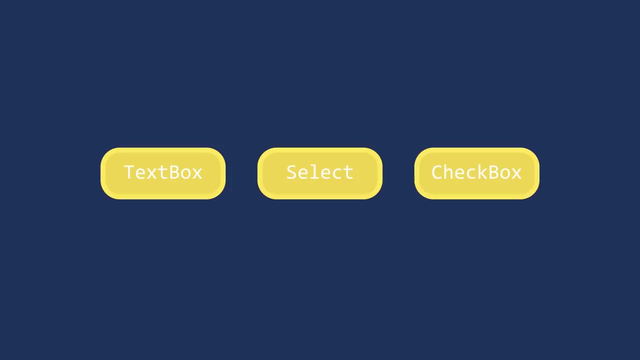 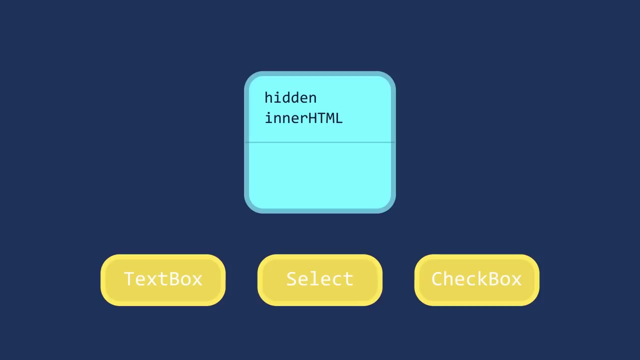 that allows you to eliminate redundant code. Here's an example. Think of a HTML element like text boxes, drop-down lists, check boxes and so on. All these elements have a few things in common. They should have properties like hidden and inner HTML and methods like click and focus, Instead of redefining all. 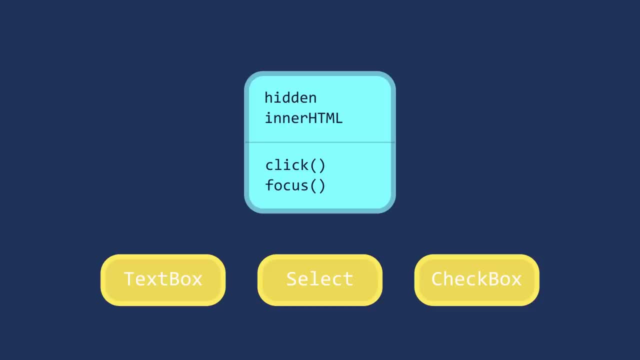 these properties and methods for every type of HTML element. we can define them once in a generic object, call it HTML element, and have other objects inherit these properties and methods. So inheritance helps us eliminate redundant code. And finally, polymorphism: Poly means many. 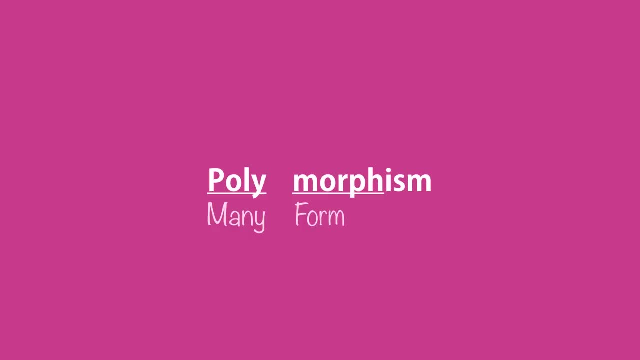 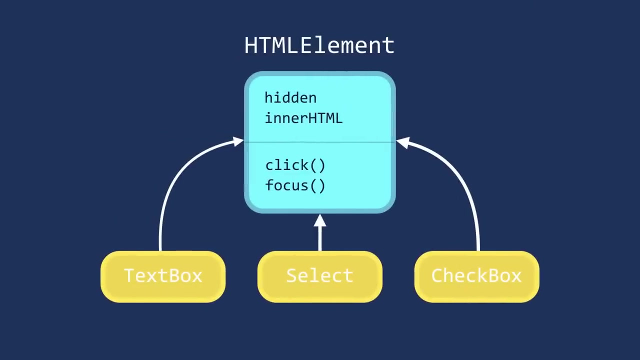 morph means form, So polymorphism means many forms. In object-oriented programming, polymorphism is a technique that allows you to get rid of long if-and-else or switch-and-case statements. So back to our HTML elements example. all these objects should have the ability to be rendered on a page, But the way each 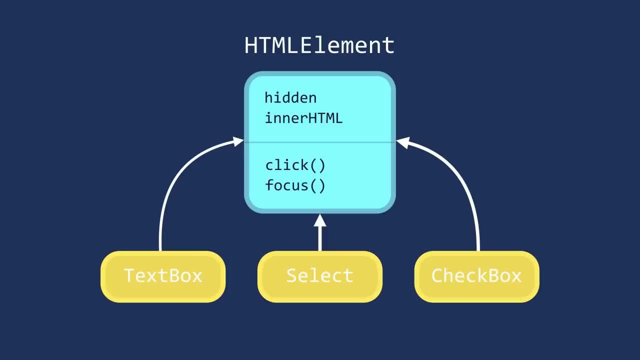 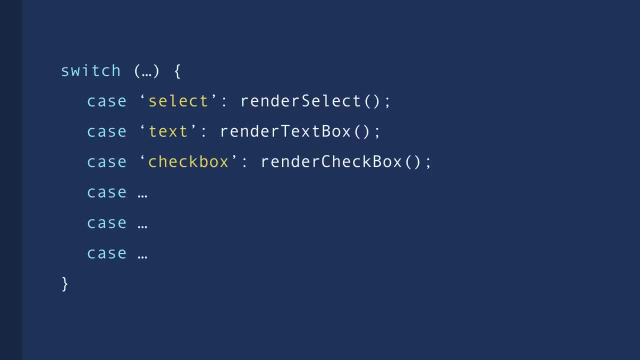 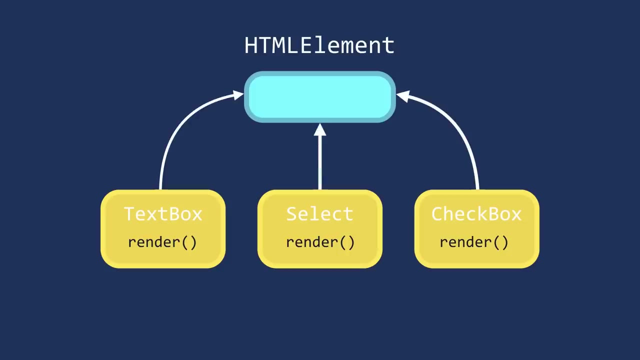 object is rendered is different from the others. If we want to render multiple HTML elements in a procedural way, our code would probably look like this, But with object orientation, we can implement a render method in each of these objects and the render method will behave differently depending on the type of the 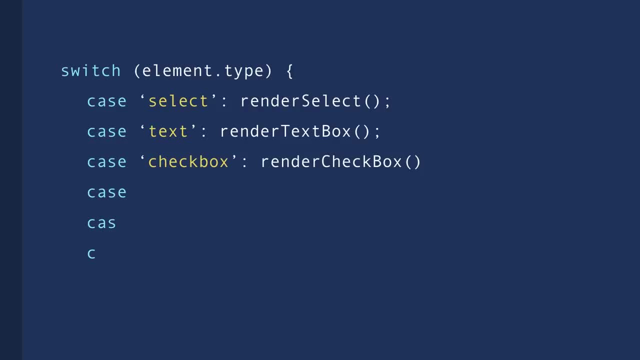 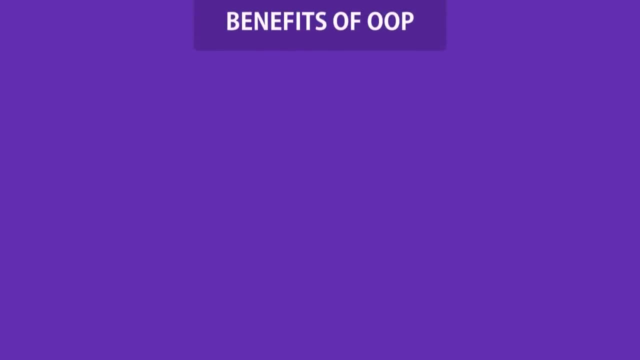 object we are referencing. So we can get rid of this nasty switch-and-case and use one line of code like this. You will see that later in the course. So here are the benefits of object-oriented programming. Using encapsulation, we group related variables and functions together and this way we can reduce. 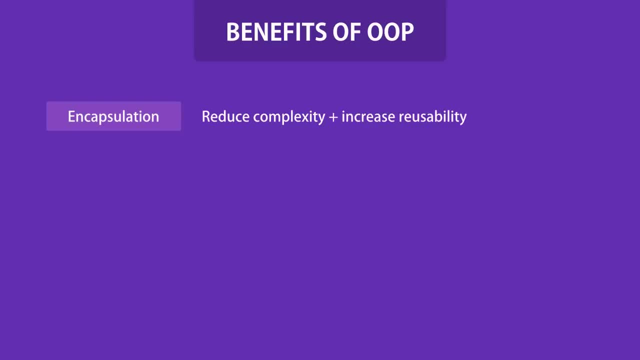 complexity. Now we can reuse these objects in different parts of a program or in different programs. With abstraction we hide the details and the complexity and show only the essentials. This technique reduces complexity and also isolates the impact of changes in the code. With inheritance we can: